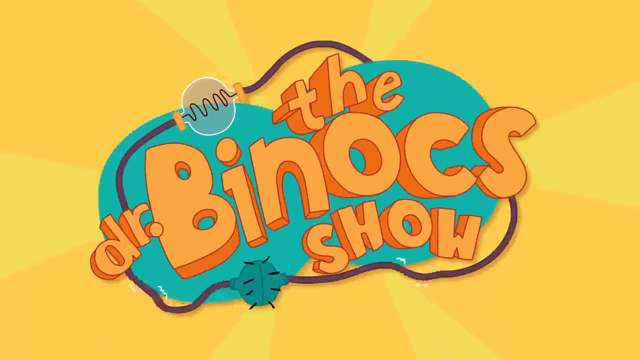 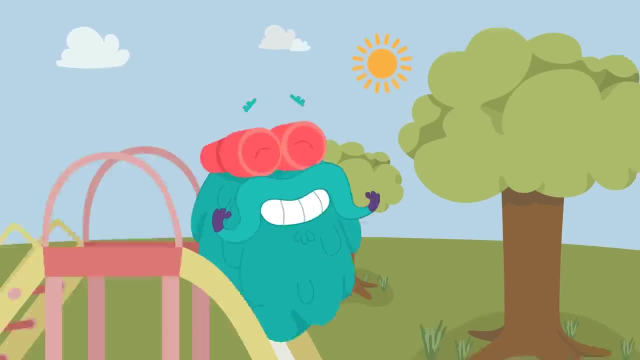 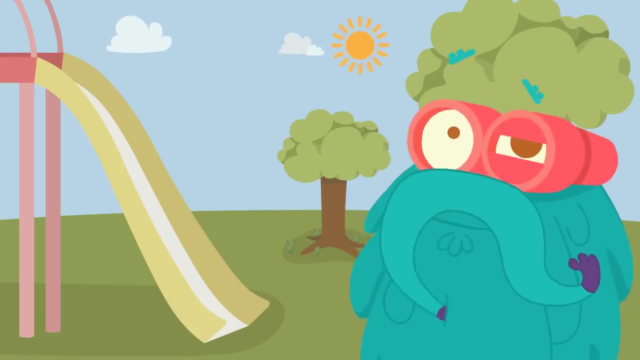 Hello friends, how's it going today? Weeeeee, So what's up? Hey, ever wondered what energy is? Well, it is the ability to do work. Wanna know more about energy? Come on then, zoom in. Energy can be found in our body. 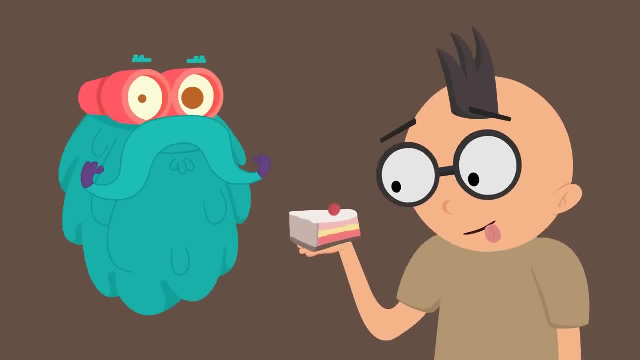 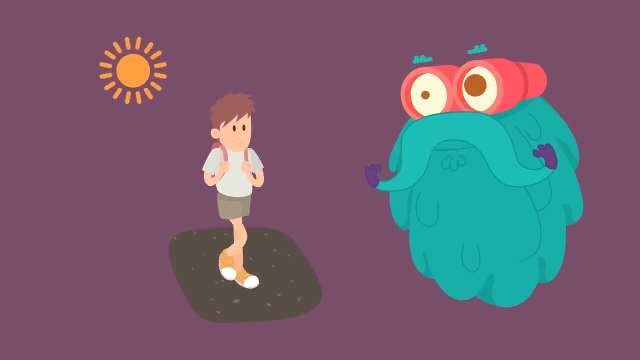 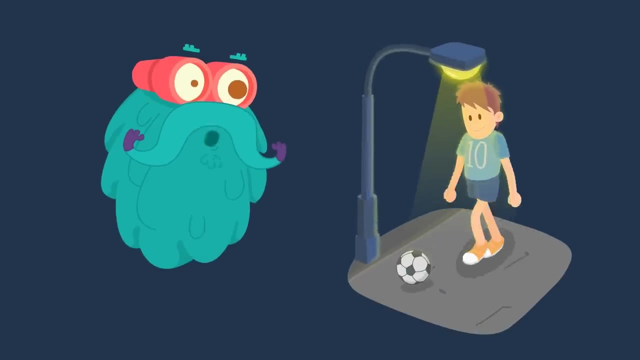 Energy can be found in a number of forms. When you eat, the body breaks down the food and gives you energy to work and play. When you go to school, you receive the sun's energy in the form of heat and light, And while coming back from playing, the street lights use electrical energy to give you light. 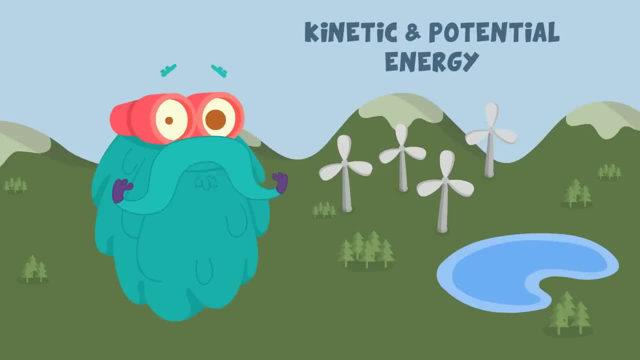 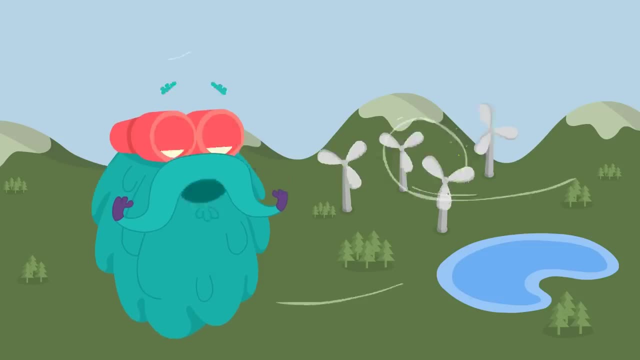 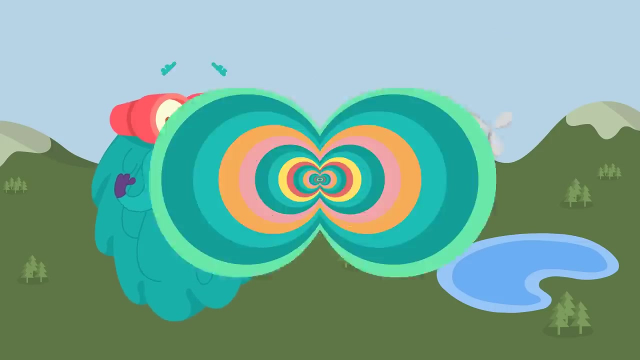 Kinetic and potential energy are the main forms of energy. Kinetic energy is the energy that is in motion. Feel the air around you. That is kinetic energy. That's because it is moving. Potential energy is the energy stored inside an object. 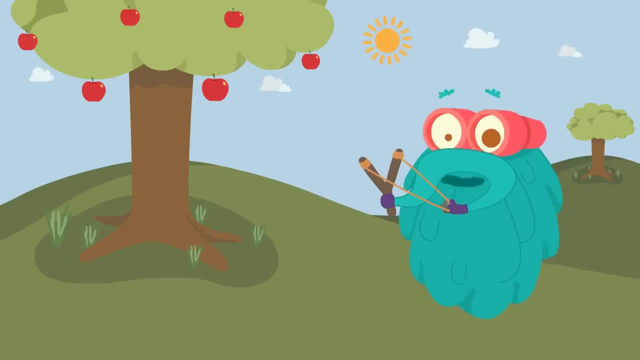 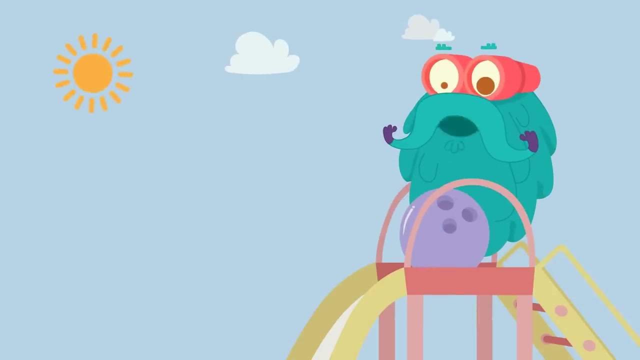 If an object is not moving and is still, it means that it has potential energy in it. It is known to have potential energy Because if it is released, it would do a lot of work. Hey, watch this. See this ball. 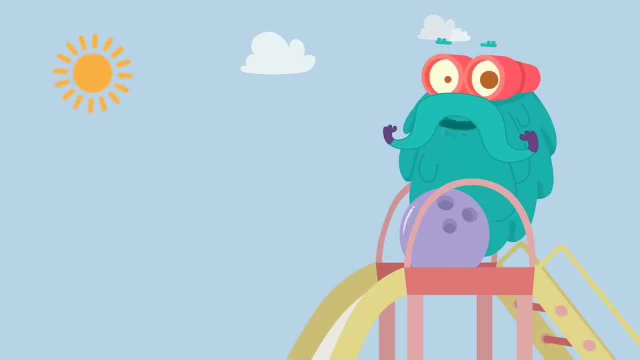 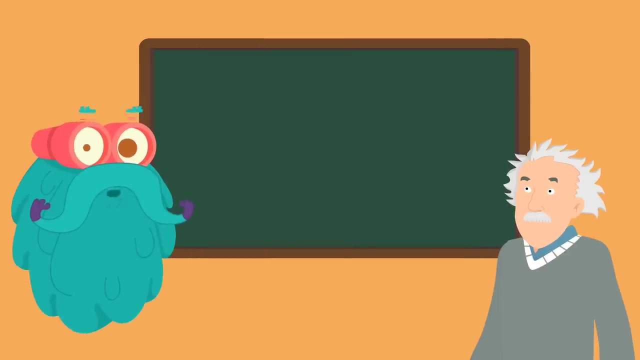 Right now, this ball has potential energy in it. This means that there is energy stored inside this ball. Let's push this now. See the ball rolling. Well, now it has kinetic energy in it. Hmm, so I am going to tell you something that you must remember for the rest of your lives. 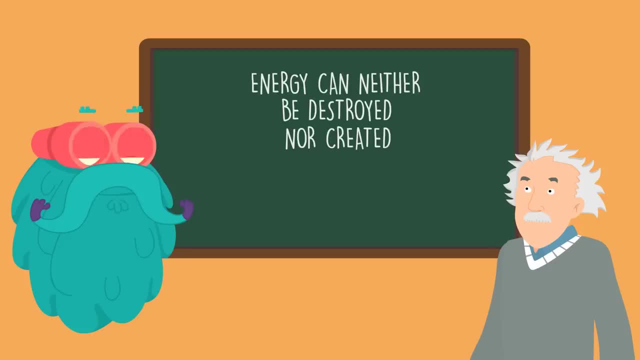 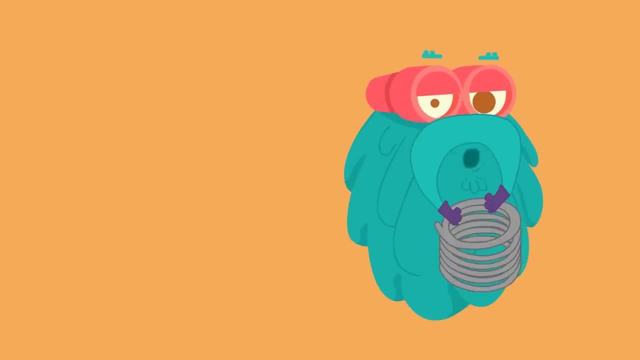 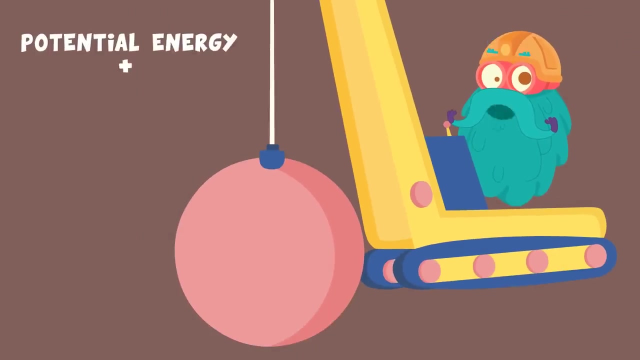 Energy can neither be destroyed nor created, But it can transform from one form of energy to another, Just how potential energy transforms into kinetic energy, Mechanical Energy. If an object has both potential and kinetic energy at the same time, it is known as mechanical energy.